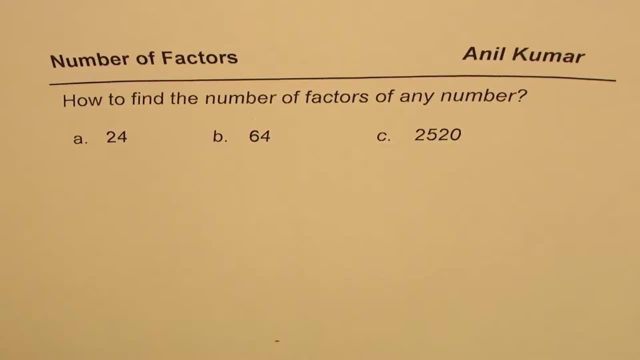 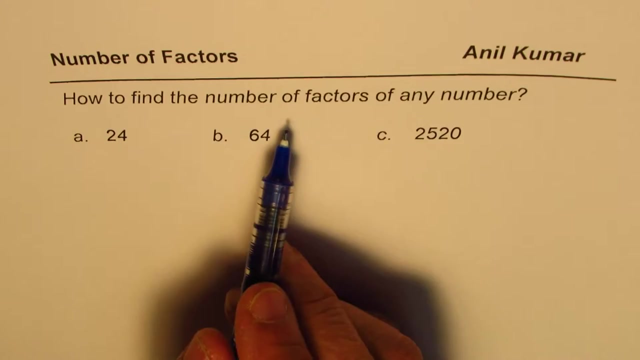 I'm Anil Kumar, sharing with you an excellent question on finding number of factors. In this video, I will actually share with you a way to find all possible number of factors for any number, howsoever big it may be. We'll begin with small numbers and then find number of factors for this. 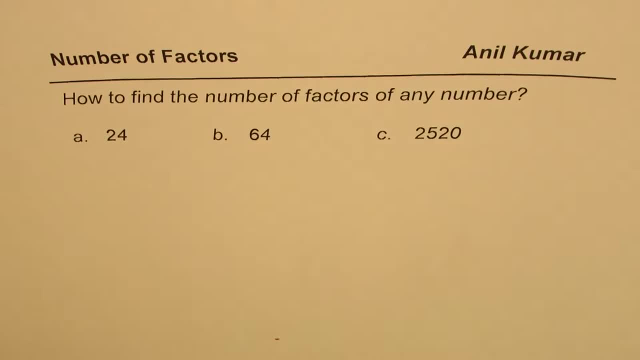 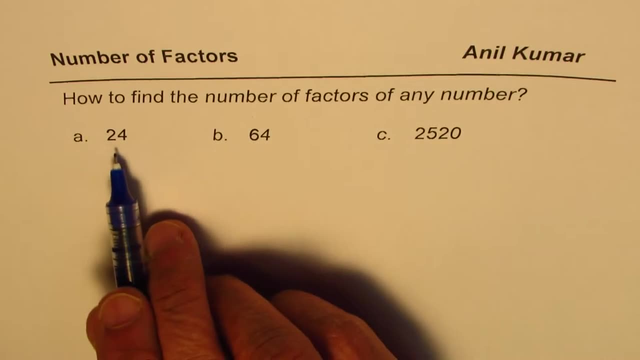 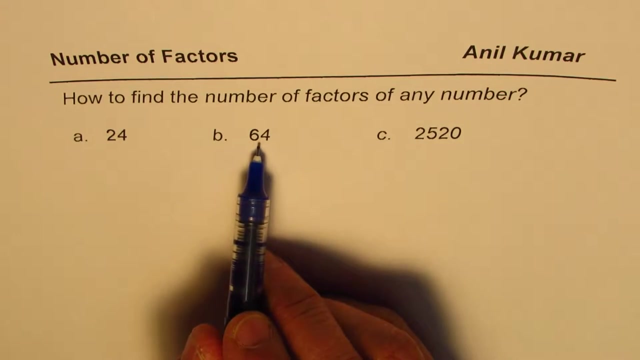 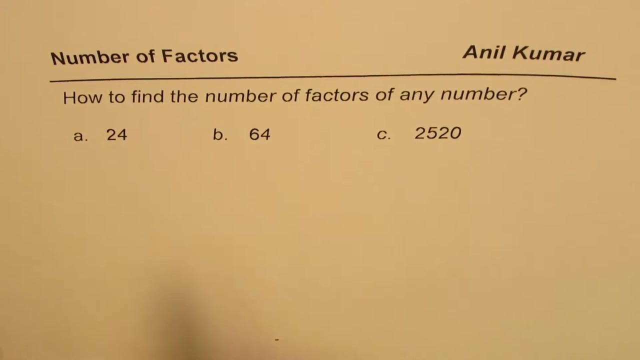 number 2520.. Now that was given to me by my student and to appreciate the concept, I've taken up two smaller numbers. So let's find how many factors 24 has, how many factors 64 has and how many factors will 2520 have. So as we learn few concepts to find factors, we could do a rainbow. 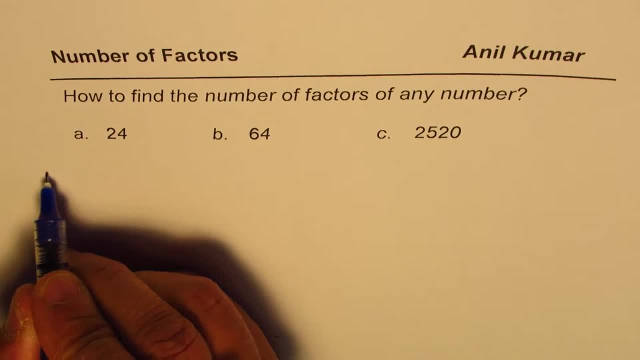 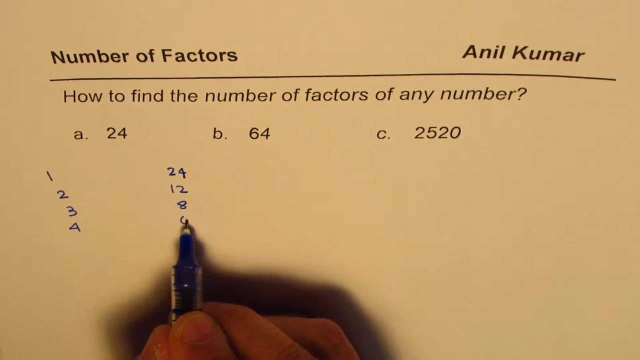 kind of a structure. 24, we know, is like 1 times 24 is 24, correct. 2 times 12 is 24, perfect. 3 times 8 is 24, 4 times 6 is 24, and then 6 times 4, so these numbers repeat. so we have 1, 2, 3, 4, 5, 6, 7, 8, so that 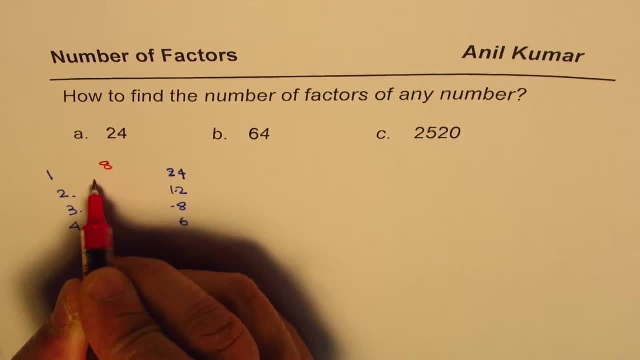 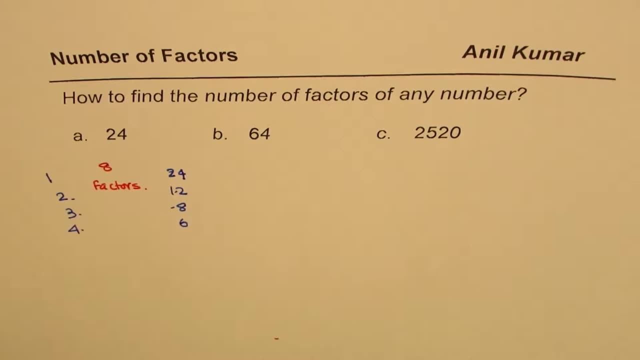 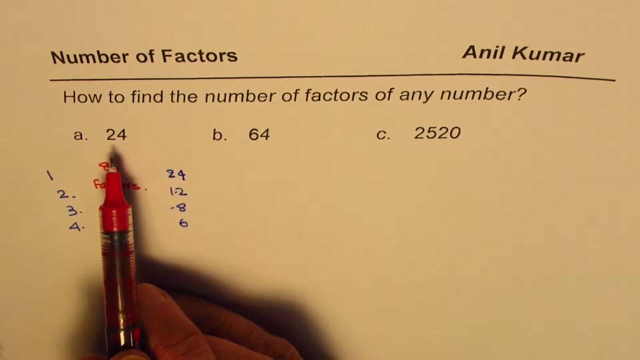 gives us 8 factors, right, so just 8.. 8 factors, perfect. so we found by listing out all the factors, and this is a good process, but it works only when we have small numbers like 24 or so right 2 digit numbers it can work well. 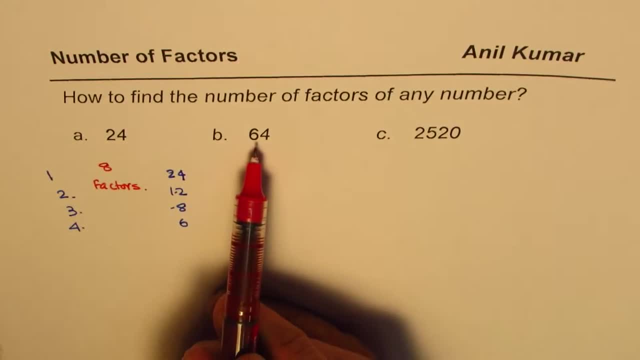 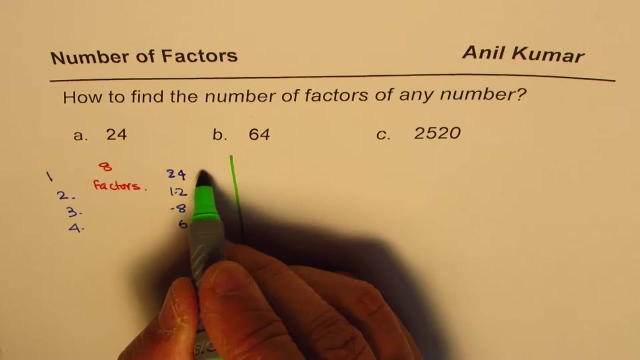 Well, here's another technique which I will show you, and this is kind of unique and we'll use it for 64. so what I will do in this case is I'll find the prime factors for this right. So we'll do prime factors. So I use this process of 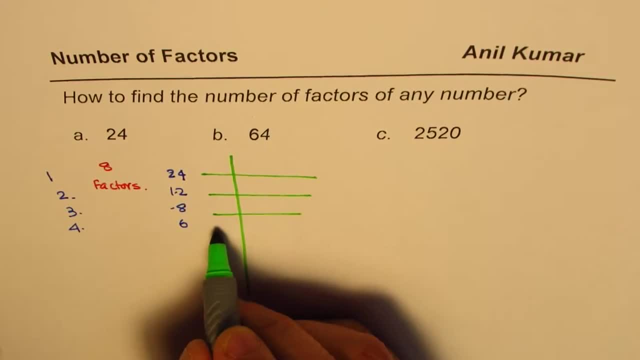 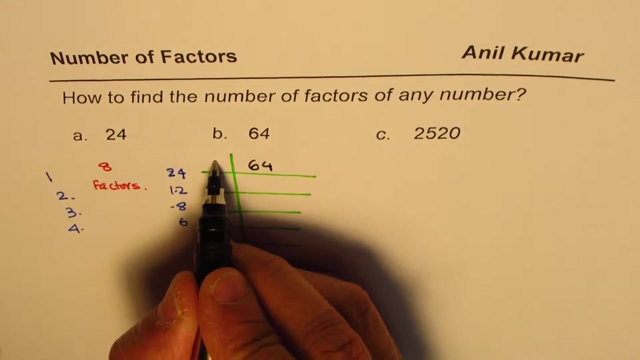 ladder division kind of thing, right? So we'll use this ladder division and then we'll find all possible factors of this one. So how do we do it? We'll keep on dividing the 64 by small numbers, right? Of course not 1, but we can do 2.. So when I divide 64 by 2,, 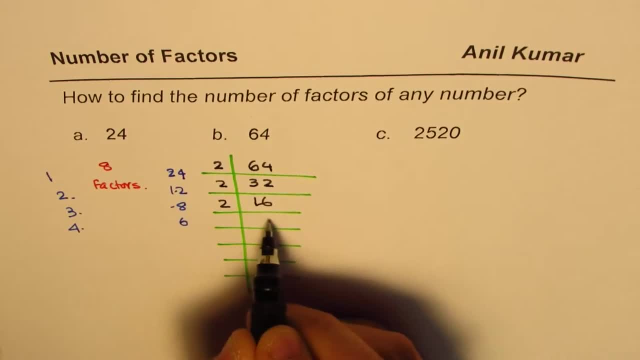 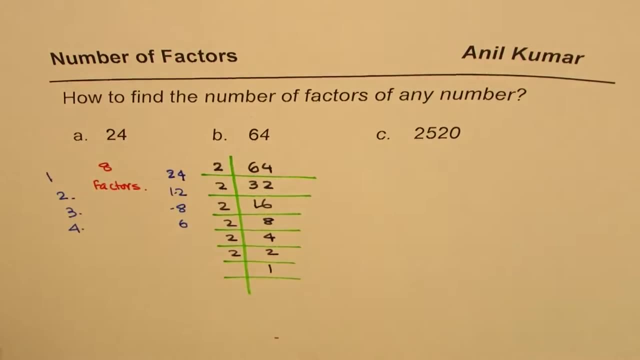 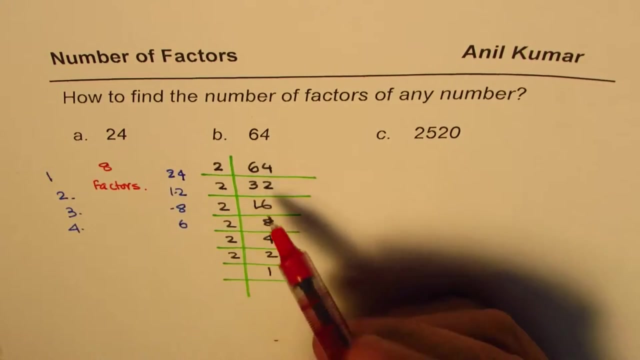 I get 32.. Then again by 2 gives me 16.. Again by 2 gives me 8.. Again by 2, 4.. And this 2. And then again by 2, 1.. Good job, So you can see. we have all the factors listed. in this fashion It gives. 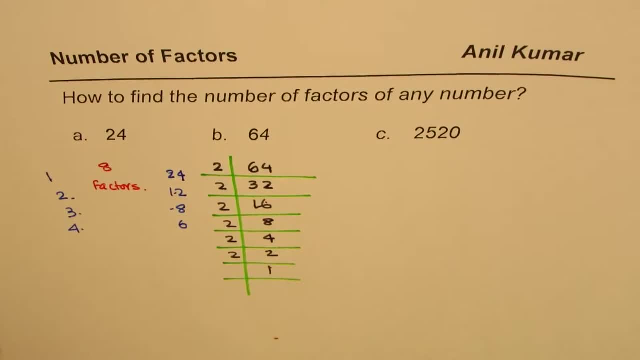 me 1,, 2,, 3,, 4,, 5,, 6,, 7 factors. So we have 7 factors. Do you see that? 7 factors? So we found total number of factors For 64 are 7.. Now what should we do with 2,, 5,, 2,, 0? That's a huge number, right? So let me try. 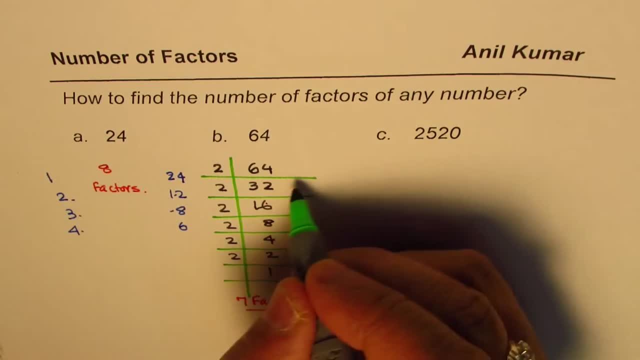 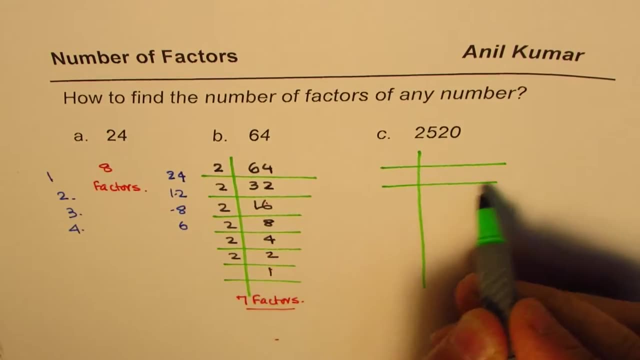 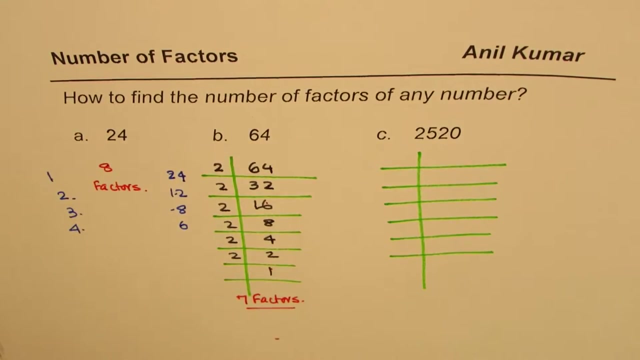 this out and see what really happens, right? So we'll try this process out and then see can we count right? So let me just try this out. This is a beautification of what we are going to do and gives me some time to think, right? So how should I go about? So I don't know really. how to do it. So let me try this out. So let me try this out. So let me try this out. So how should I go about? So let me try this out. So let me try this out. So let me try this out So. 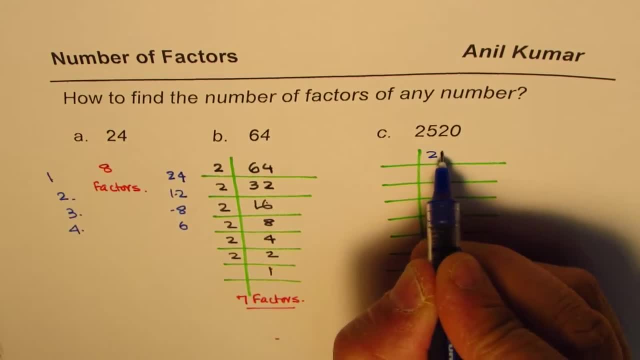 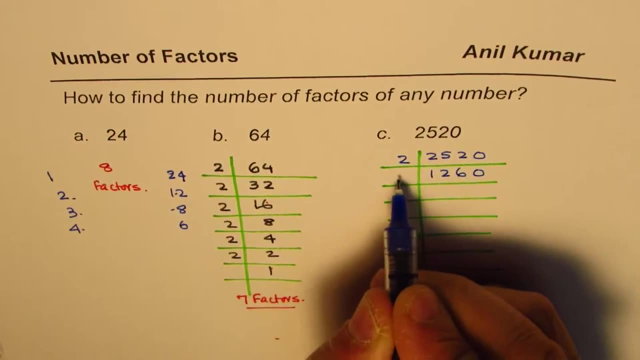 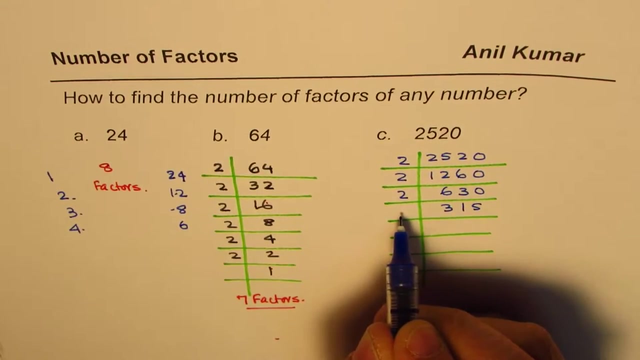 I'm thinking about it. So we have this number: 2, 5, 2, 0. So let's again divide by 2, which is 1, 2, 12 is 6, 0. Then again by 2, 6, 3, 0. Just do half of it: 3 and 1, 5.. And then, well, this: 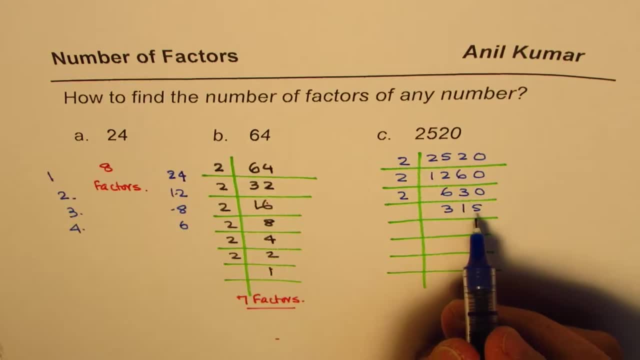 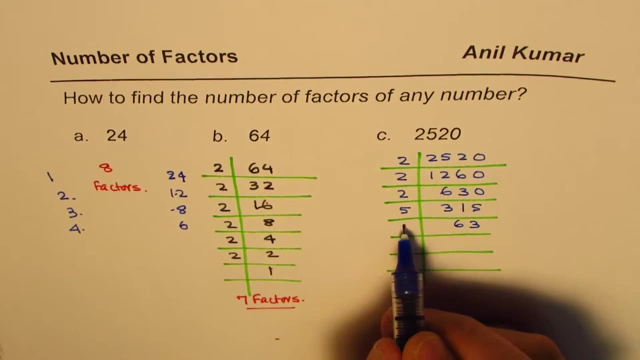 time. 2 is not going to work, but 5 can work. okay, So we'll do 5.. 5 times 6 is 30 and 3.. And 63 means 3 will work, So we'll do. 5 times 6 is 30 and 3.. And 63 means 3 will work, So we'll do. 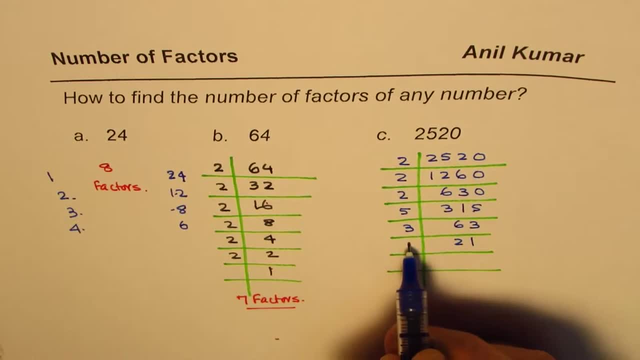 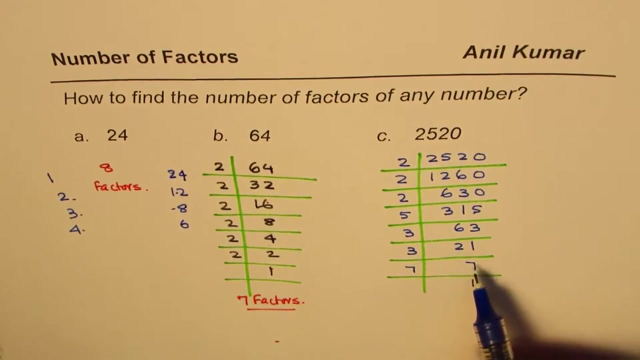 will work. So we have 21, and then again 3 will work, which is 7, and then let me write 7 and 1.. Well, so we have all the list of factors here. Is it possible for you to count them and then get the answers? So you say 1,, 2,, 3,, 4,, 5,, 6,, 7,, 8, and well, this seems. 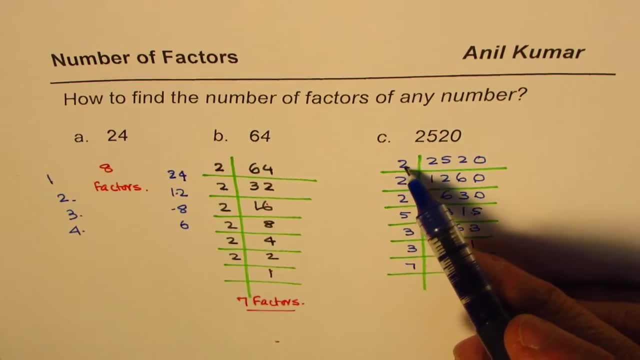 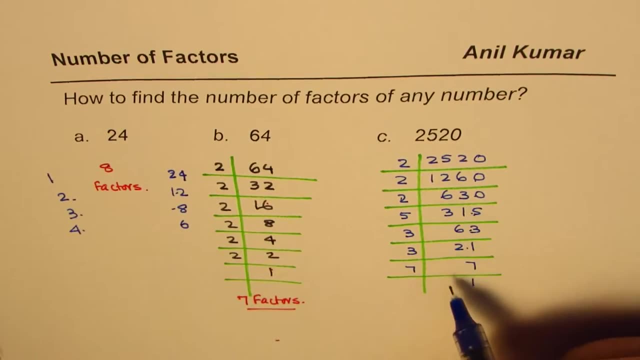 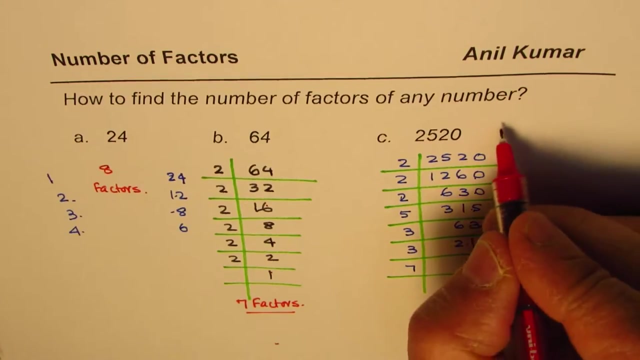 to be same. You said 9 and 10, 11.. Like this, you can kind of count and you will not be very sure whether you got the right numbers or not. It requires a lot of work here, But here is a trick. So let us learn the method. This is extremely important method. So what? 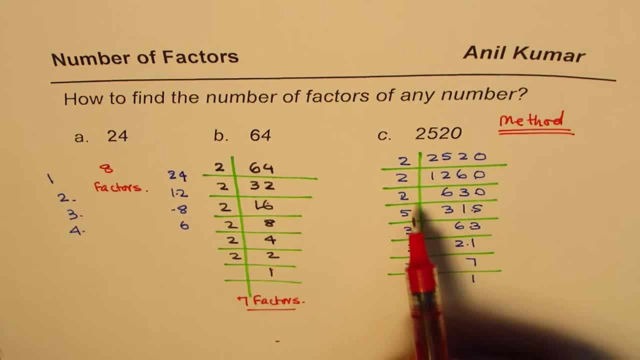 you notice here is that I could write 2,, 5,, 2, 0 as product of these numbers, Now 5. How many 2s do I have? Let's see. So what I have here is, as far as the 2s are concerned, we have. 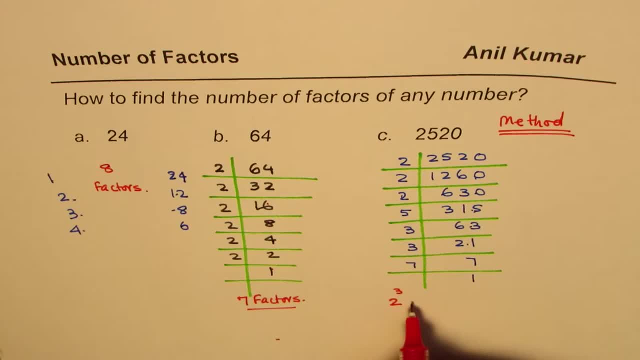 1, 2, 3.. So three factors of 2 times how many 5s? 1. How many 3s, 2. How many 7s? Just 1, right. So what we do here is we list out all the factors and how many times do they occur. 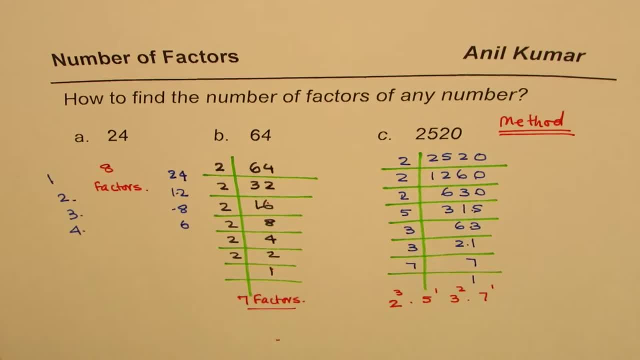 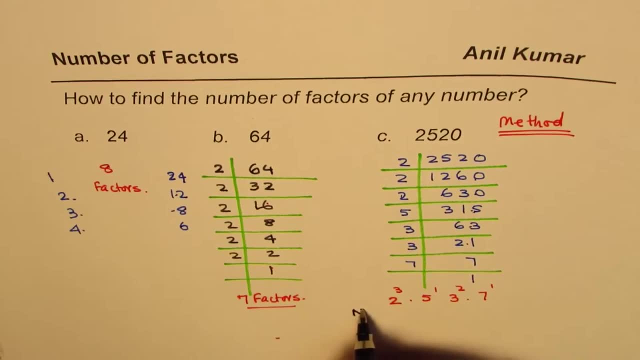 when we do this kind of prime factorization. Now to find the total number, let's call that total number to be n. n is actually related with these exponents. So if it is 3,, I write 3 plus 1 times. If it is 1,, I write 1 plus 1.. And if it is 2,, I write 2 plus 1.. And if it is again 1,. 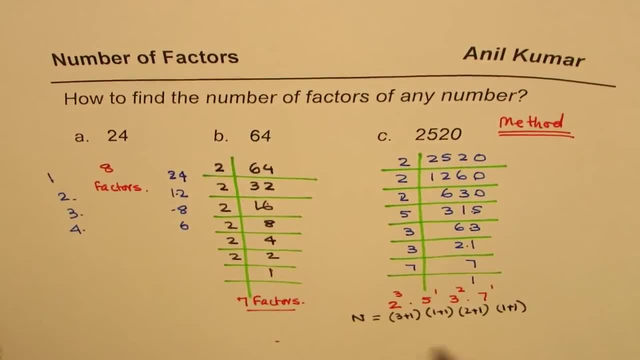 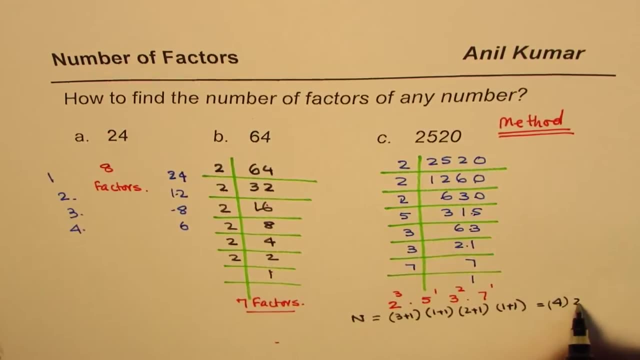 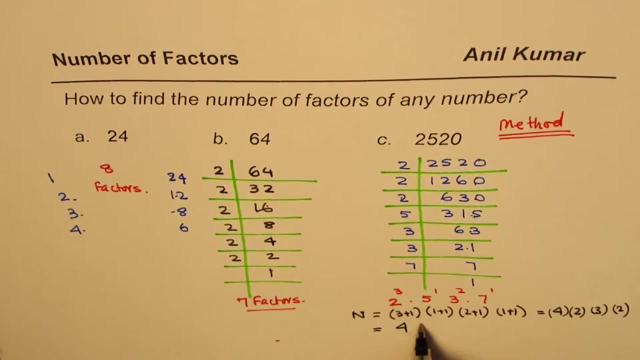 I write 1 plus 1, right? So that's gives me total number. So it is 3 plus 1 is 4, and then times 2, and then times 3, and then times 2.. That should be my answer. 4 times 2 is 8.. 8 times 3 is 24.. Times 2 is 48.. So what I get here is 48.. 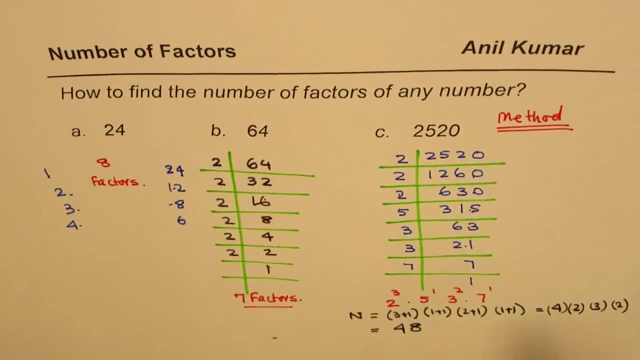 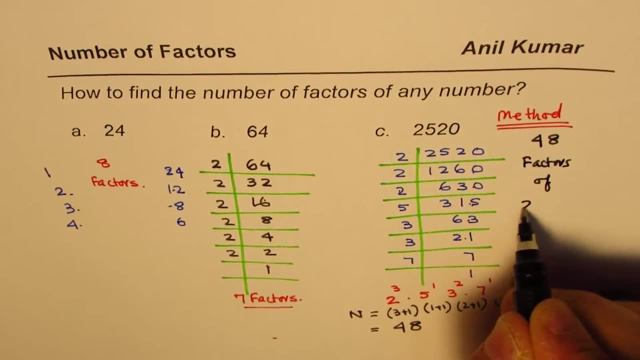 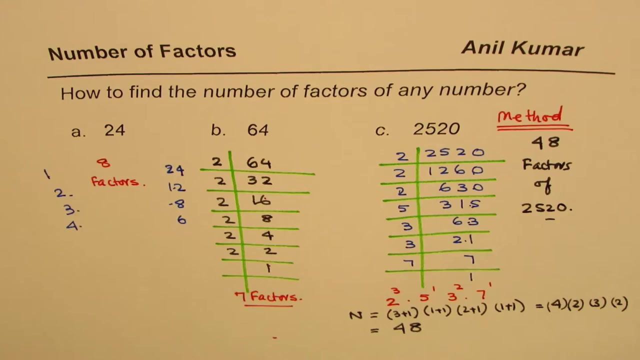 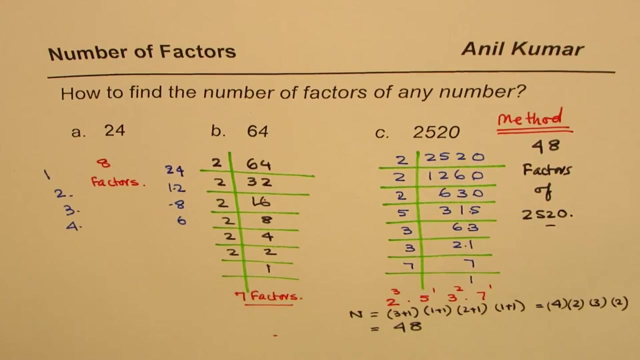 So my answer for this is that we have 48 factors of 2520.. Now, I may be right, I may be wrong, but that's what I get. Now, how do you confirm that this rule works? Well, we have two correct results here, which we counted. Let's check with. 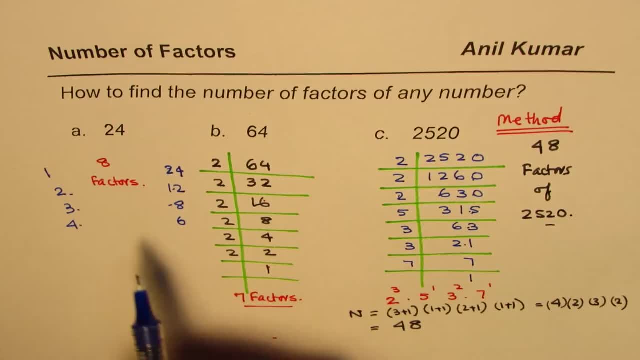 those results. Okay, that's a good idea. So if I do prime factorization of 24, what do I get? Let me redo all this process, okay, So I'll again make this kind of a tree. I mean, okay, I have enough space here, So let's do it.